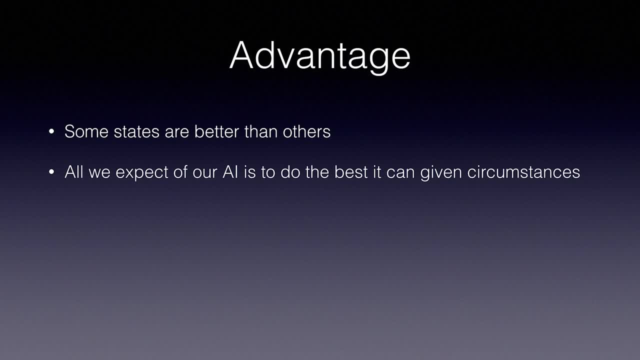 With a less intelligent baseline like this, our agent can take a really good action in a bad situation and still get punished for having a low reward. Advantage rewards anything better than expected for the state. To calculate the advantage, we simply take the Q value for each state and action. 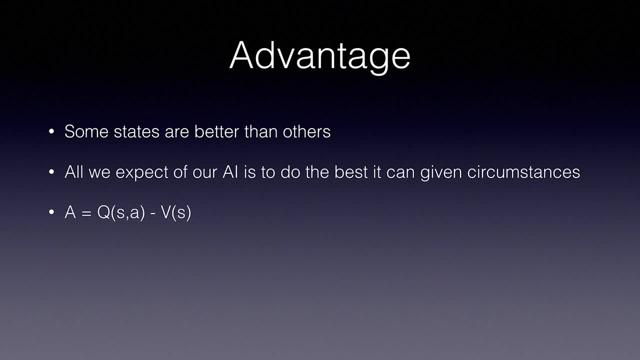 That is the calculated return for the action taken minus the estimated value of the state which comes from our network. If the returns on an action are better than the expected value of the state, we increase the probability of taking that action, And if the returns are worse than expected, we decrease the probability. 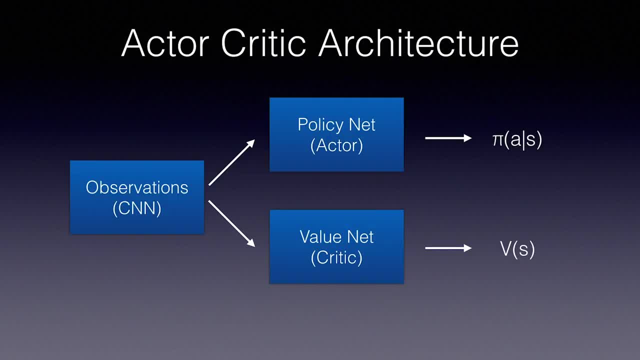 Now the next step toward getting cutting-edge reinforcement learning results is the actor-critic architecture. We're going to use a neural network with two outputs: a policy head and a value head. The policy head outputs probabilities for taking each action. The value head outputs a single number: the value of the current state. 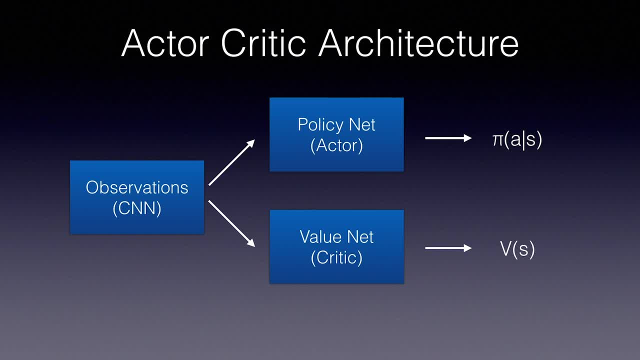 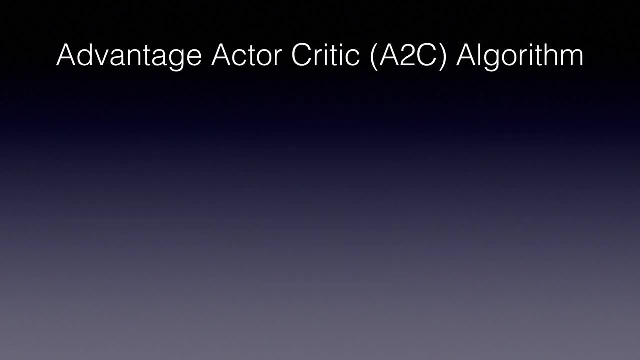 The predicted value is then subtracted from the actual returns of the action to obtain the advantage And we scale the policy gradient. Alright, let's take a look at the basic advantage actor-critic algorithm, also abbreviated as A2C. First, we initialize the network parameters, theta, with random weights. 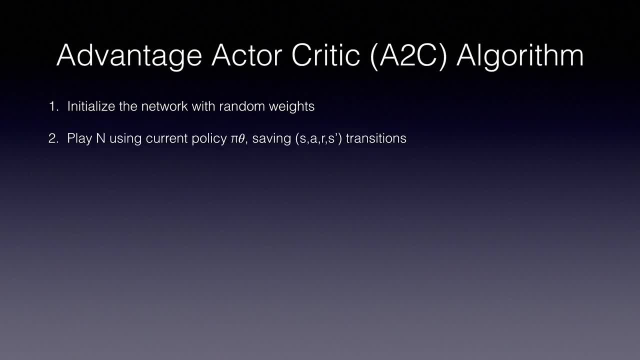 2. Play end steps in the environment using the current policy, saving state action-reward transitions. 3. Set r to 0 if we reach the end of the episode. Otherwise, set r to the value of the action. 4. I equals t minus 1 all the way to t start. 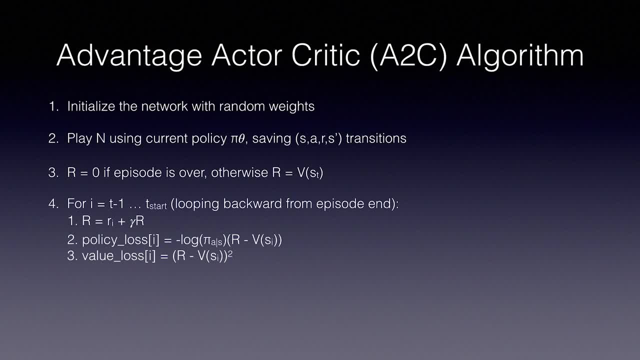 Now we're looping backwards from the end of the episode. r equals the reward from this time step plus gamma times r. The policy loss is the negative log probability times the advantage. Value loss is simply the mean squared error of the actual return calculated minus the value of the state that our network estimated. 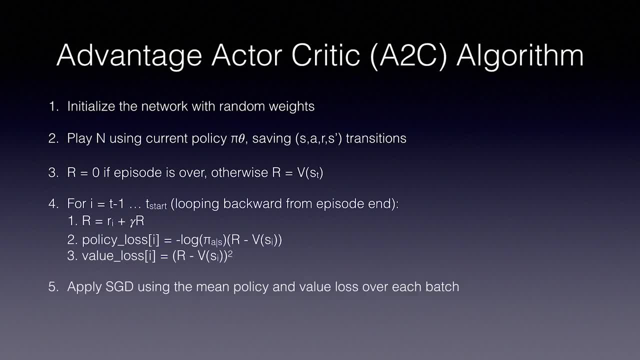 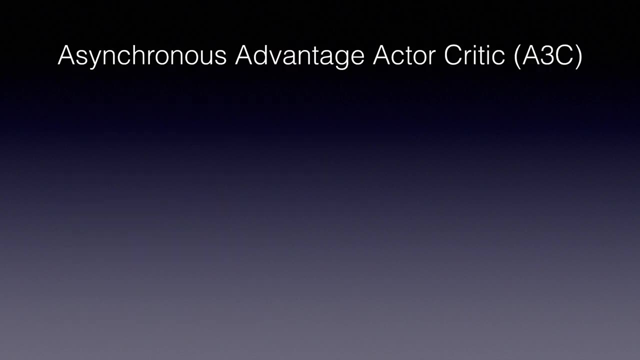 Step 5. We apply stochastic gradient descent using a mean policy and value loss over each batch, And 6. We repeat from step 2 over and over again until the learning has converged. Alright, now let's take a look at the asynchronous advantage: actor-critic, abbreviated A3C. 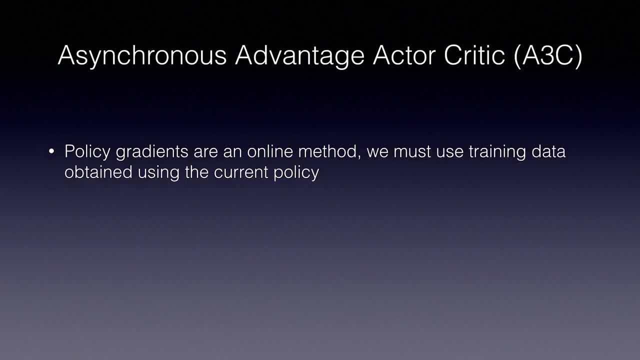 Policy gradients is an online method, which means we must train on data obtained from the current policy. Yet to keep our training data independent and identically distributed, IID we still need a large buffer of transitions to train on. The solution is to run multiple environments in parallel to obtain large amounts of training data from a single policy. 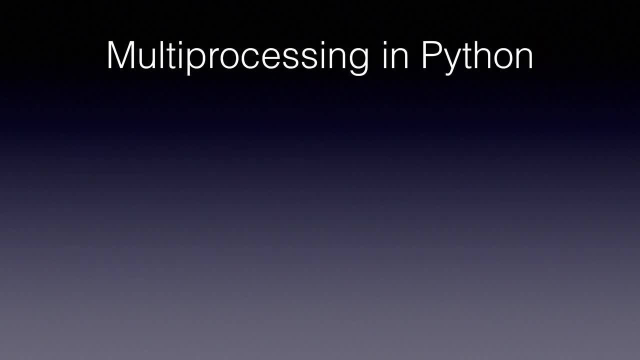 This is much faster with multiprocessing, which we can do in Python. mpq is a thread-safe FIFO first-in, first-out queue for transporting training data to the network. mpprocess runs a piece of code in a child process with methods to control it from the main process. 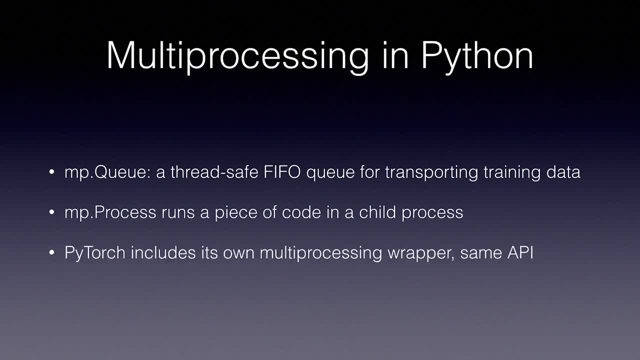 pyTorch includes its own multiprocessing wrapper, torchmultiprocessing, which properly handles tensors and shared memory across both the CPU and GPU, And the API is exactly the same as Python's multiprocessing API. The goal of this series is to build step-by-step from the basic concepts towards the most advanced reinforcement learning algorithms. 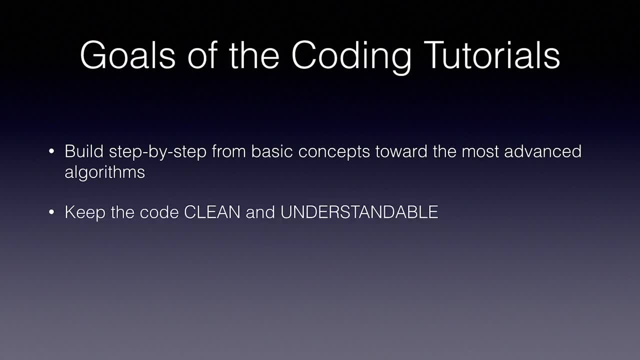 mpq is a thread-safe FIFO first-in, first-out queue for transporting training data to the network. My goal is to keep the code clean so that you understand it, and not necessarily to provide the absolute best implementation of actor-critic possible. In the following videos, we are going to learn how to tweak this actor-critic architecture to get the absolute best results on a variety of tasks. 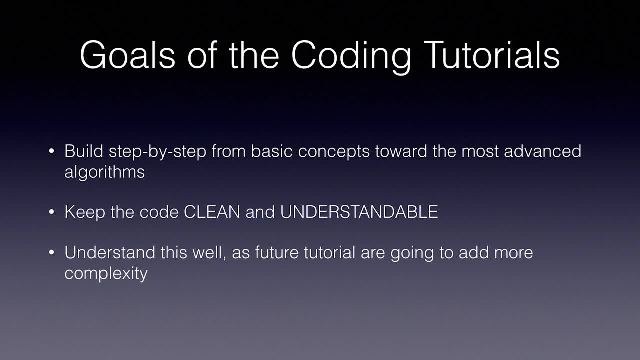 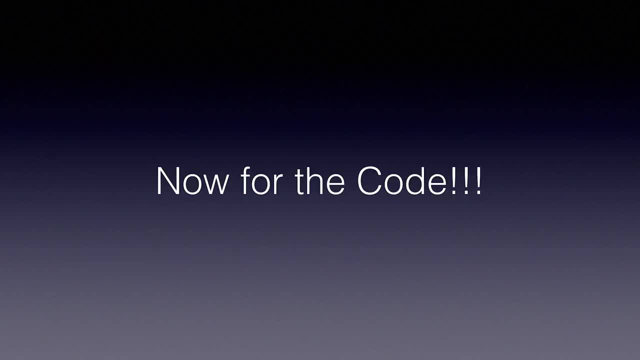 We're going to be adding even more complexity later, so be sure you understand well what is happening here before moving on. Alright, let's jump into the code. mpq is a thread-safe FIFO first-in, first-out queue for transporting training data to the network. 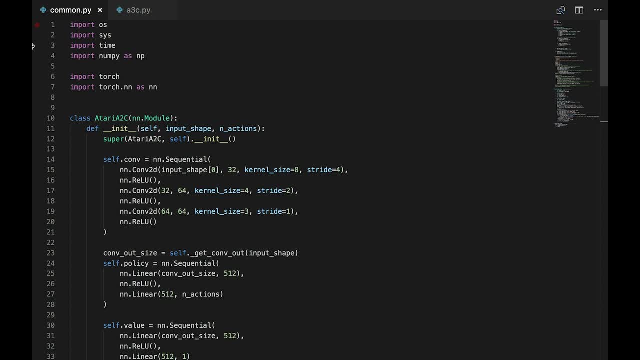 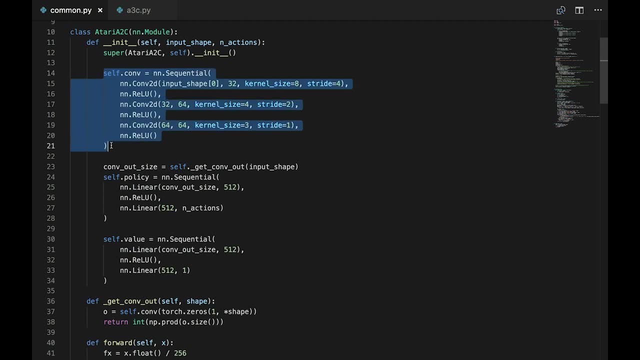 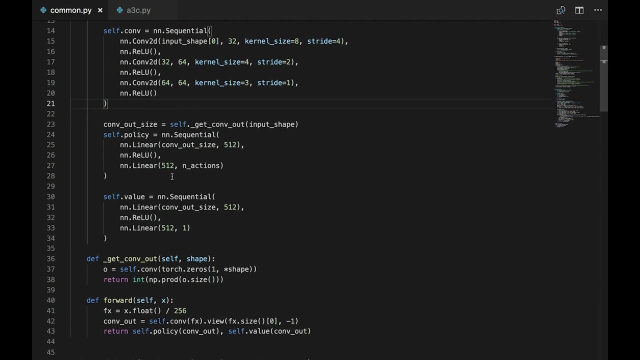 We'll start with the architecture of the neural network in the Atari A2C class. First we have the same convolutional layers as before. The output from the observation head is then split and passed into the separate policy and value heads. These each contain a hidden layer of 512 neurons plus an output. 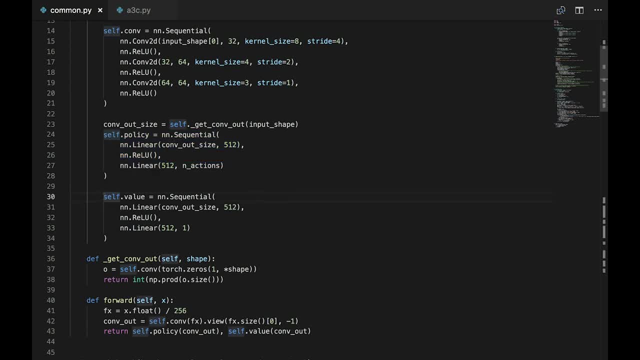 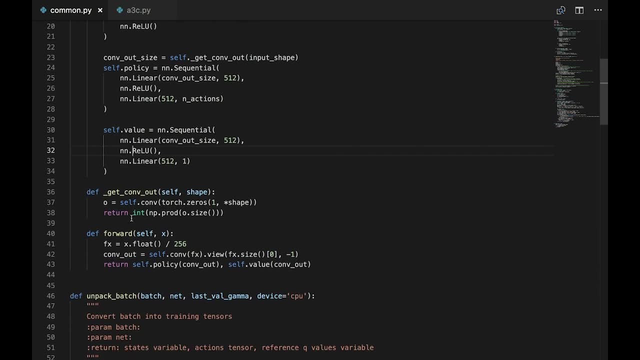 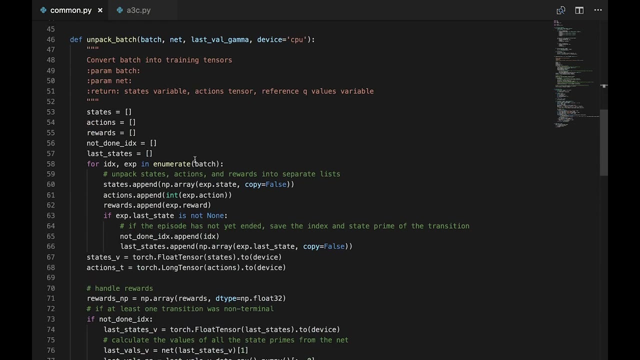 The policy network outputs logits representing the probability of each possible action. The value network outputs one value: the estimated value of the state that was input into the network. Next let's look at the unpack batch function. This returns separate torch tensors of states actions and calculated queue values of the state-action pairs. 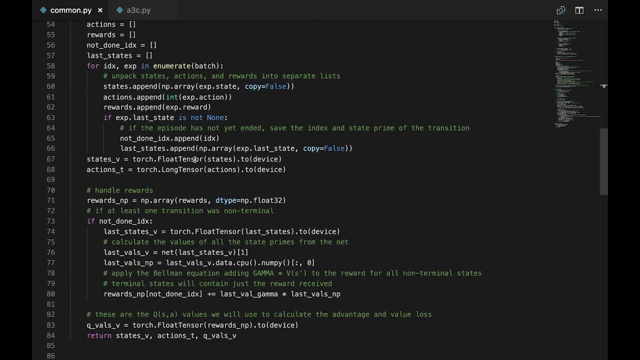 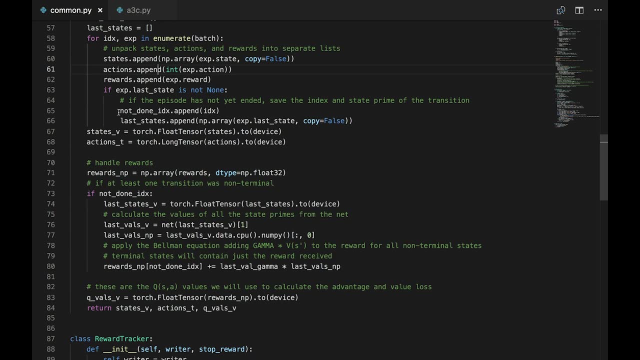 First we unpack the states, actions and rewards into separate lists. Then for each transition where the episode is not over, we need to calculate the value of state prime. So we save the index and state prime of each non-terminal transition. 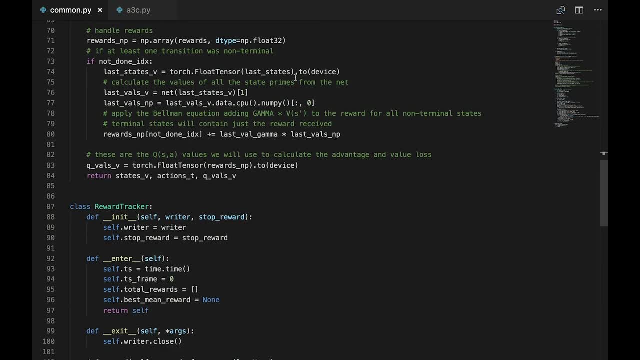 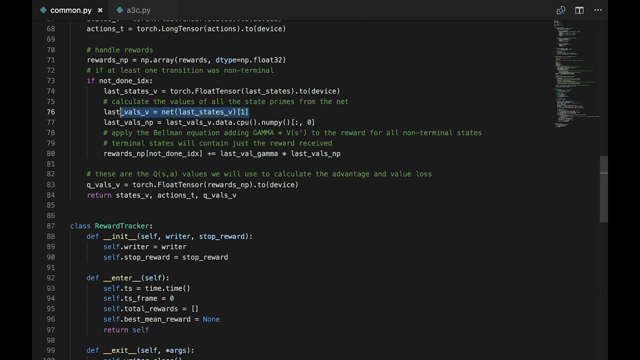 Next, let's look at the unpack batch function. For each non-terminal transition, we pass a state prime list through the network to estimate the values. If the state was terminal, the queue value is simply the reward received. Otherwise, the queue value is the reward plus gamma times the value of the state prime. 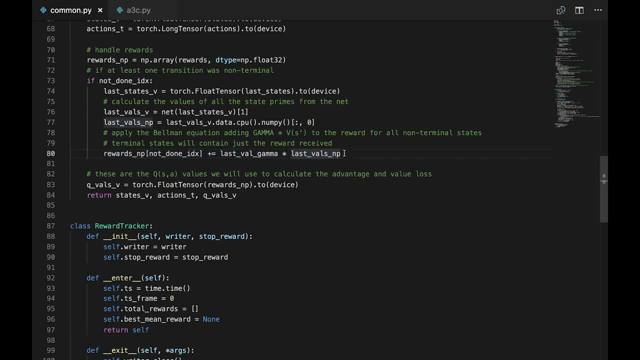 Note that, since each transition contains multiple unrolled steps, we are actually using gamma to the power of num steps. Finally, we convert everything back to torch tensors and return the states, actions and queue values. The reward tracker class keeps statistics on each episode. 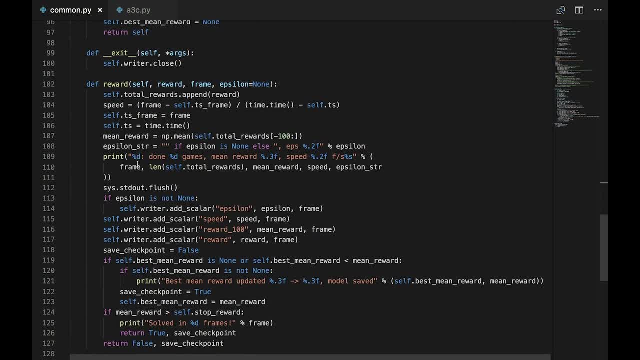 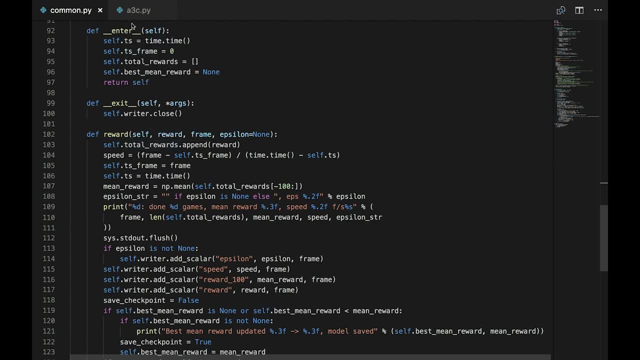 and tells us when training is finished, as well as when to save the checkpoint when we have reached the new highest-ever reward. This is the same as we used before. Now let's move on to the main A3Cpy file. At the top, as usual, we have the hyperparameters. 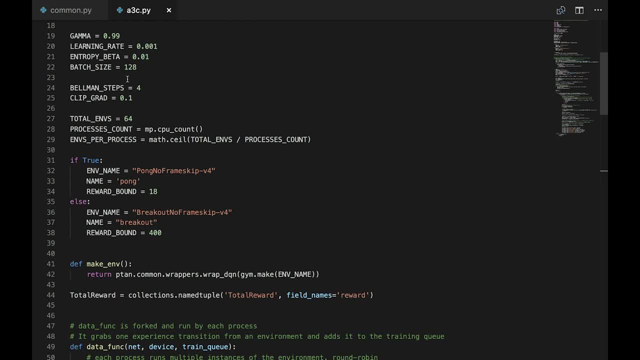 Most of these are the same as in previous tutorials. You'll recall one of the biggest problems in policy gradients is over-adjusting the policy and screwing it up. clipgrad limits the size of the update across each layer of our network at each step. 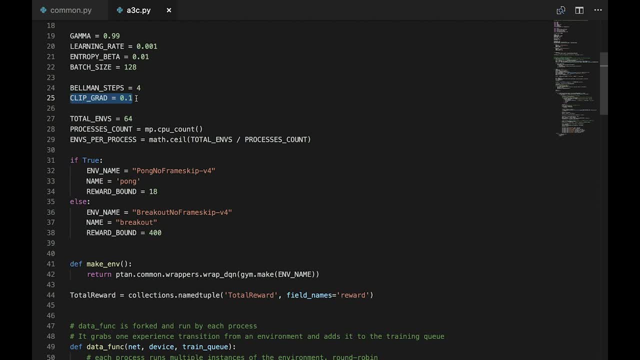 This makes training more stable. Total environments is the number of environments that we are going to be running in parallel. Process count is the number of cores that your CPU has and is looked up automatically through the multiprocessing library. Environments per process is the number of environments that we are going to be running in parallel. 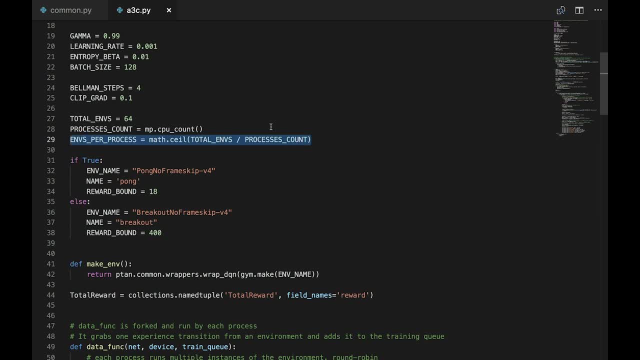 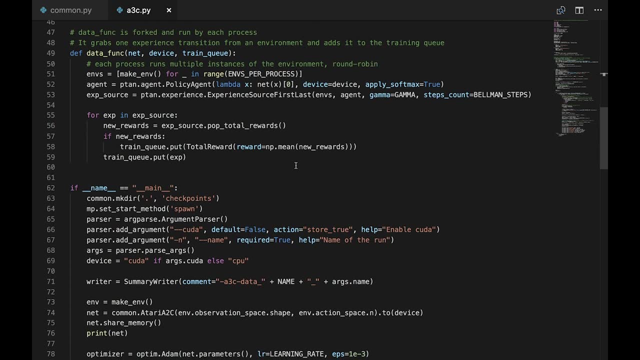 that will be run inside each child process. Moving down data func is a function that is run inside each process. It takes a reference to the neural network, the device- either CPU or GPU- and a reference to the training queue. It generates a specified number of environments. 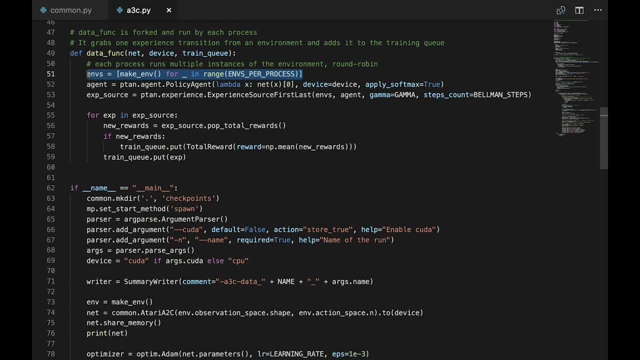 that the agent will be playing and reporting data on. Then it simply plays episode after episode, appending each translation to the queue until the process is stopped. Every time an episode is complete, we output the total rewards from that episode. Now on to the main program. 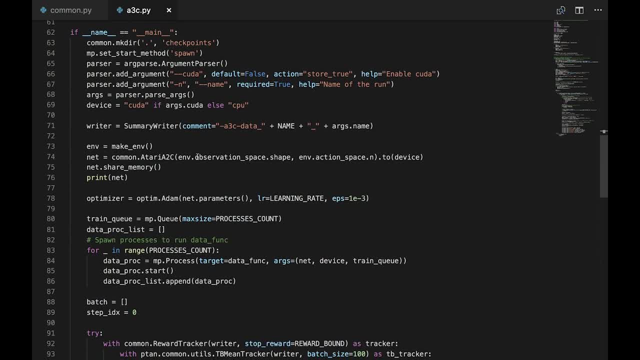 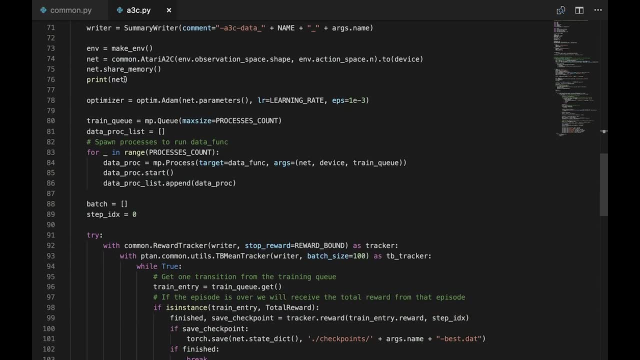 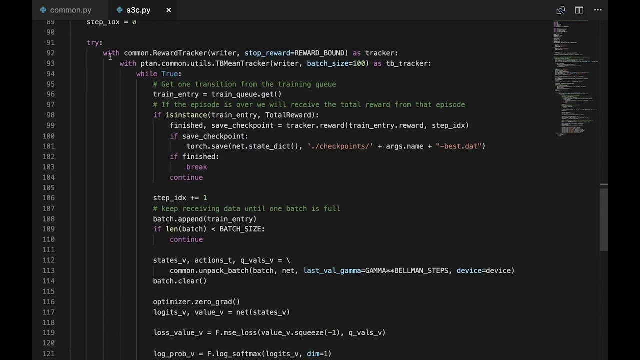 We initialize the neural network in the training queue. We spawn an instance of data func for each processor in our computer. We enter a try block. This means that if we encounter any error, the training will be aborted, but the cleanup section under the finally block will still run. 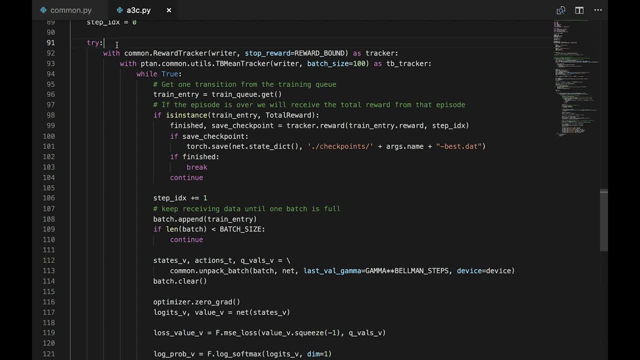 We're going to track the total reward of each episode. We're also going to track a moving average of the statistics over 100 episodes. Now we enter the training loop. We pluck one training entry from the queue If it is an instance of the total reward class. 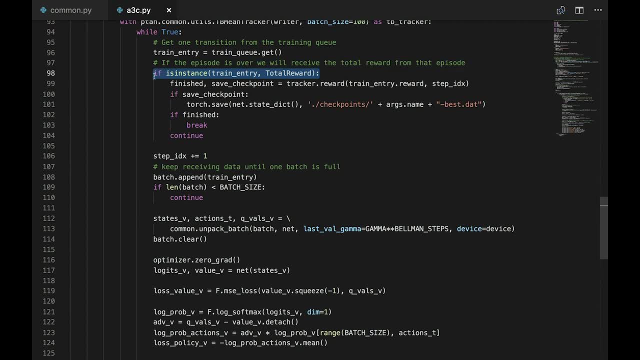 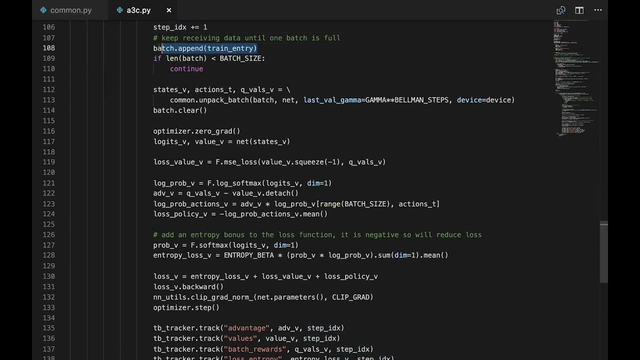 we track the total reward and conditionally save a checkpoint. We append training entries to the list until we have a complete batch. Then we unpack the batch to get a list of states, actions and queue values. We clear the batch to empty the list. 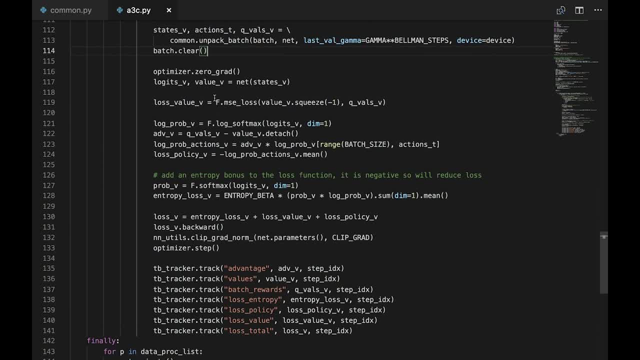 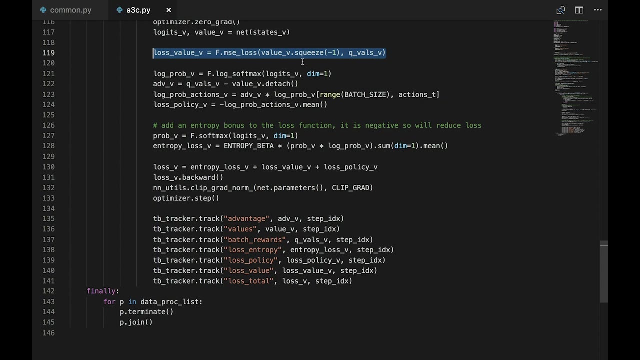 We zero out the gradients in the network. We input the batch of states into the network and get back batches of logits and values. The value loss is calculated by a simple mean squared error. The logits go through a softmax and are converted into log probabilities in one shot. 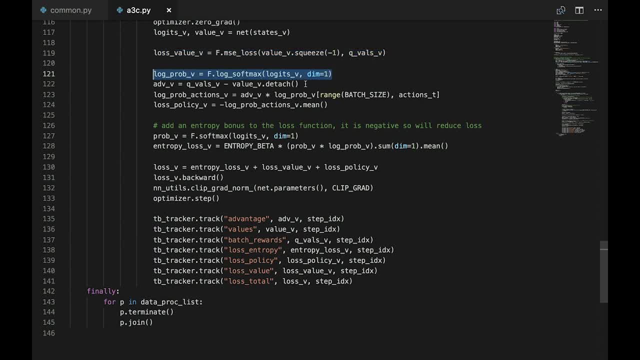 The advantage is the reference queue values we calculated, minus the estimated values from the value network. The policy gradients- negative log probabilities- are scaled by the advantage. Policy loss is the mean gradient over the batch. As before, we are going to add an entropy bonus to the loss function. 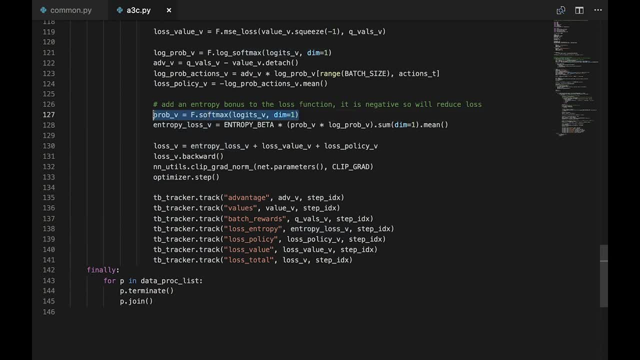 Actually, we were supposed to take the negative entropy bonus and subtract it from the loss, but the two minus signs cancel each other out When the entropy is high, and thus the network is uncertain about which action to take. this will reduce the loss. 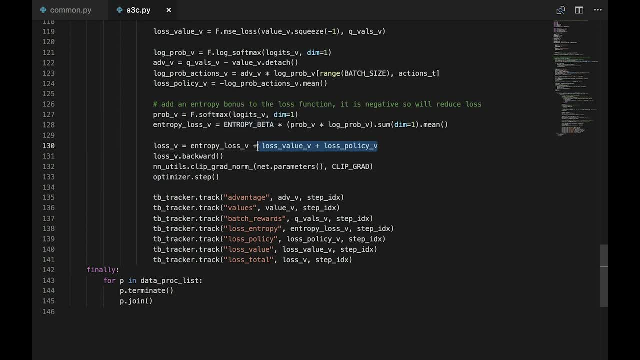 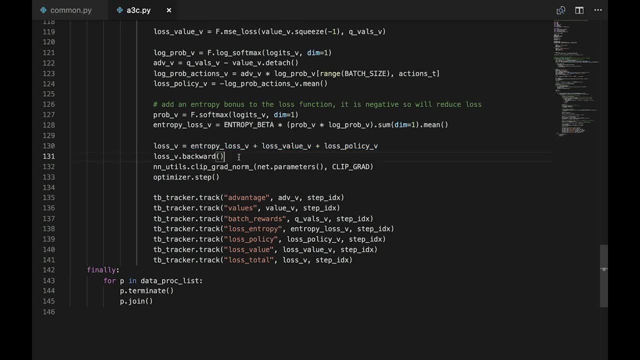 It is common in actor critic to give the policy loss more importance, such as 2x, by reducing the value loss. but we're not doing that here. We back, propagate the loss, clip the gradients to prevent large changes and then run one step of the optimizer. 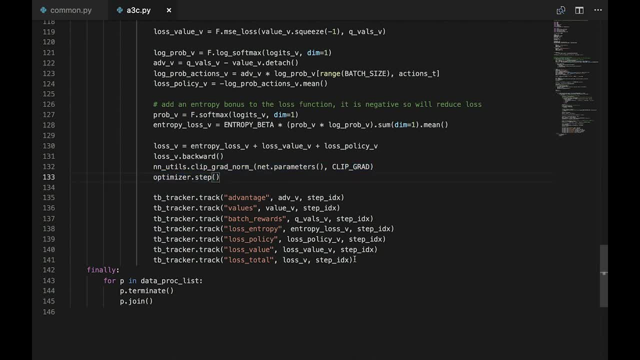 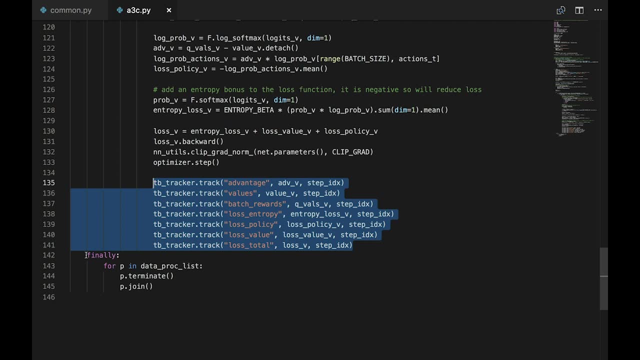 For the last part, we are simply tracking a bunch of useful statistics in TensorBoard. We went over most of them in the policy gradients tutorial. When training is done, done, the finally block performs cleanup. We send a signal to terminate each process and then wait.